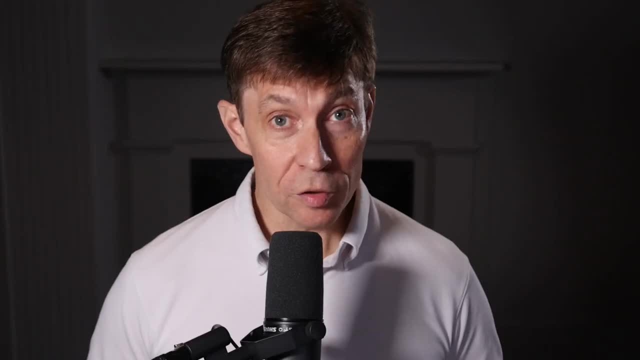 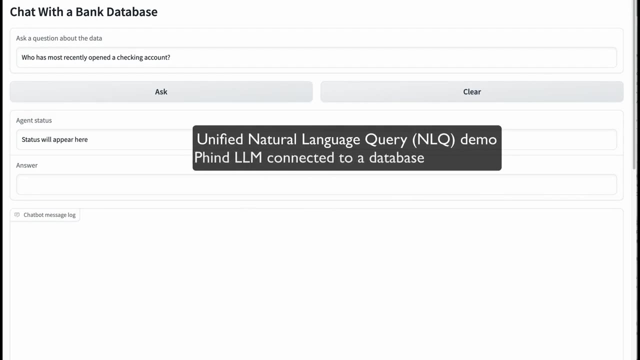 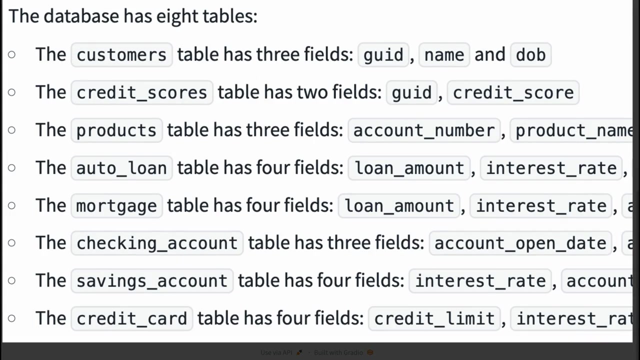 name Find optimized this model for writing code, which is what we need. Here is a working demo. The scenario is the same as episode 4, except we modified it to use Find instead of GPT-4.. Once again, we have a database consisting of tables you would expect to see in a bank's CRM. 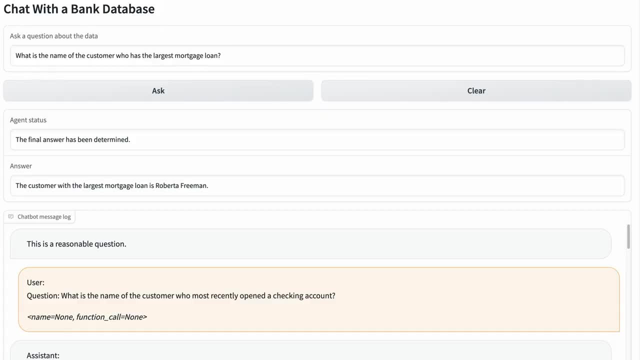 such as customers, credit scores and products. With this application, a bank manager can ask questions about the data, such as: what is the name of the customer who has the largest mortgage loan? Answering this question requires LLM agents to come up with a plan. 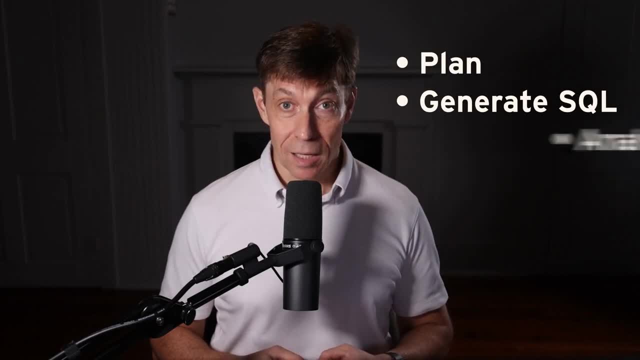 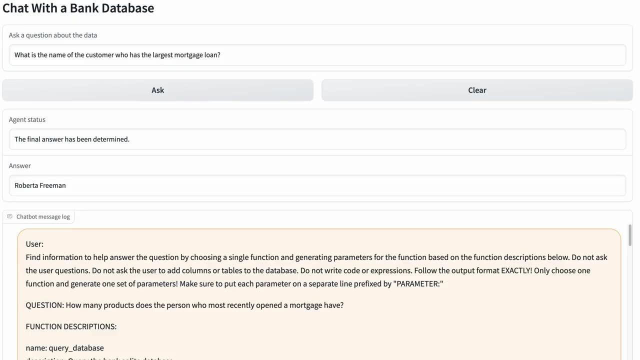 generate SQL code for getting the data and analyze it. This is a hard problem and the holy grail of business intelligence. Additionally, we made it more realistic by adding messy data. The correct answer is Roberta Freeman and the open source Find model is able to solve it. 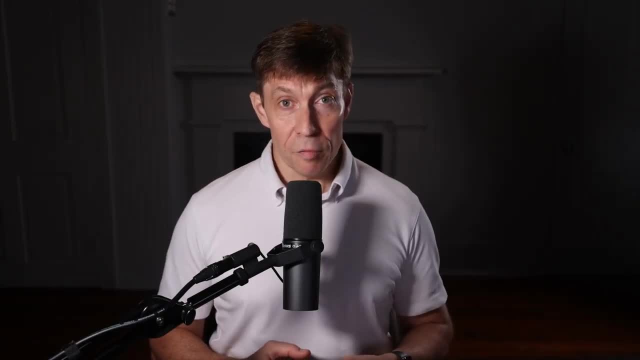 just as GPT-4 does. If you want to learn more about the OpenAI model, go to wwwopenaicom. Now let's begin comparing Find to GPT-4.. First, notice how much more efficiently Find writes the SQL code. 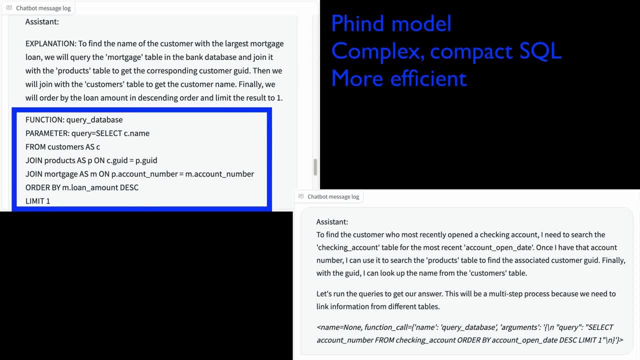 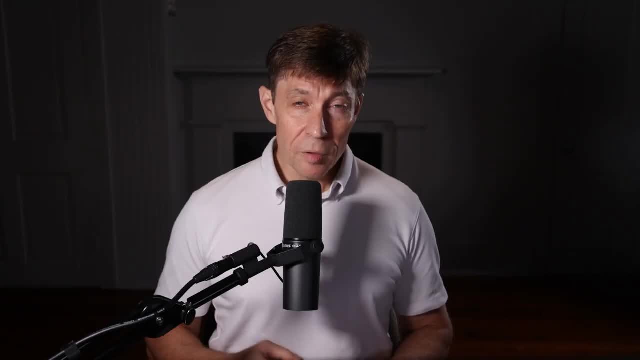 It can generate more complex single queries to answer questions, whereas the GPT-4 version generated simple queries that took multiple prompts. Subjectively Find looks almost as good as GPT-4, but we want a more objective way to compare them, So we create an evaluation framework similar to 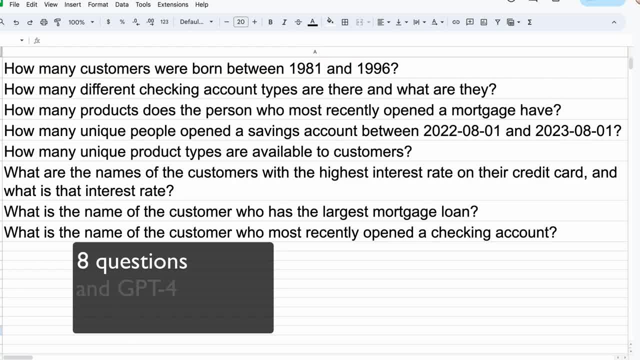 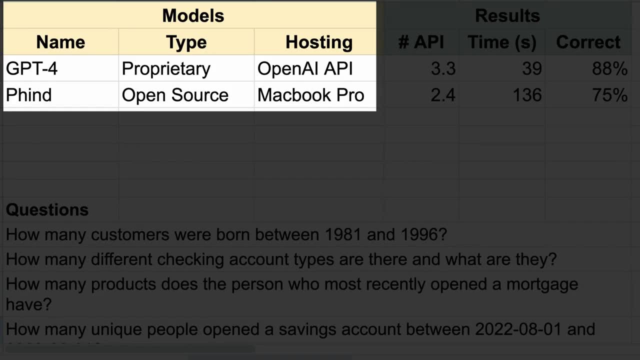 episode 6.. We started with these 8 questions and built an evaluation framework to run each through the GPT-4 and Find models 3 times and average the results. Here are the results: We are comparing the performance of the proprietary GPT-4 model hosted by OpenAI and the free, open source Find. 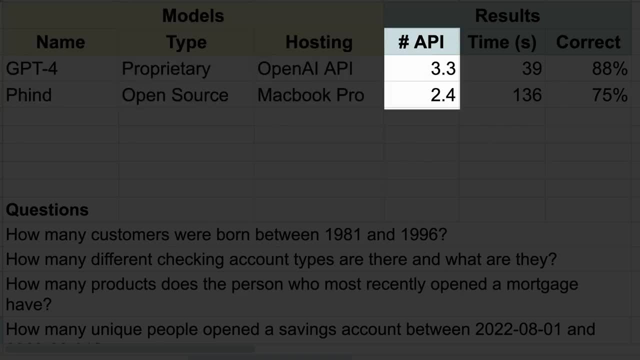 model running on my laptop. The number of API calls identifies how many requests were made to the model. Find takes fewer calls for the reason I mentioned earlier. It is better at writing the complex SQL queries. Let's look at the completion time in seconds. Find is about 4 times slower. 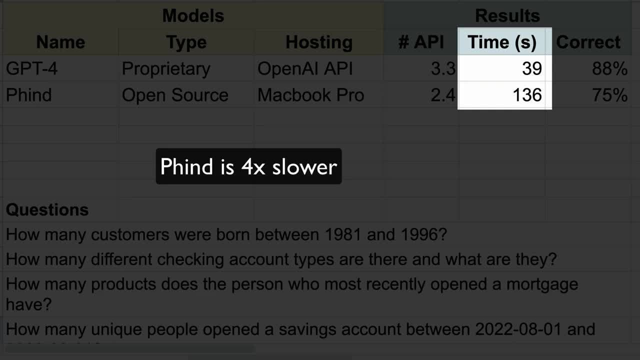 but this is more impressive than it seems. Obviously, the hardware is the biggest factor. Find is running on a $2000 consumer laptop, while OpenAI is running on Microsoft's cloud infrastructure- the best in the world. Moreover, we can significantly improve Find's performance. 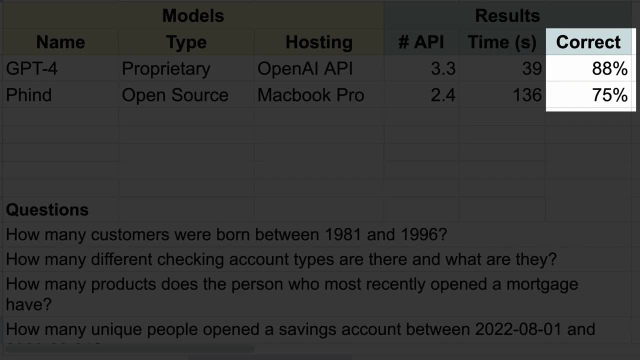 with a few minor changes. Now let's look at the most important metric: how often the models correctly answer the question. Find is running on a $2000 consumer laptop, while OpenAI is running on Microsoft's cloud infrastructure. At first glance, neither result is particularly exciting. 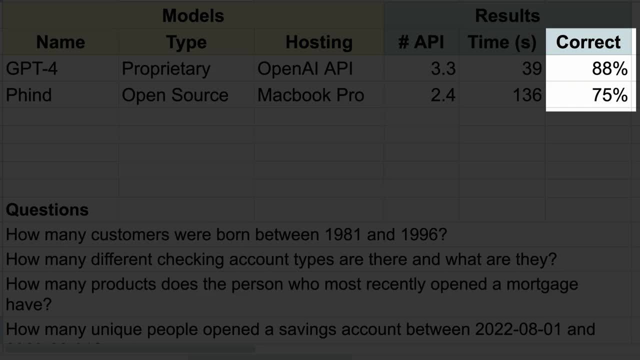 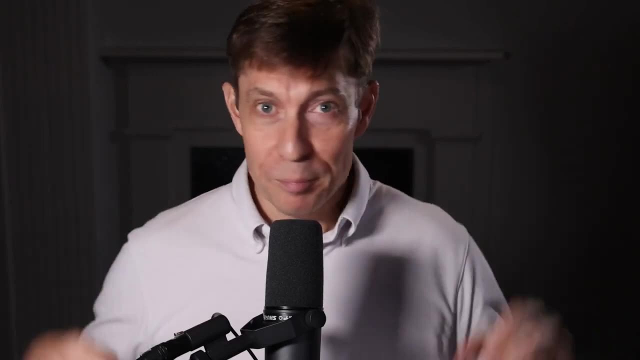 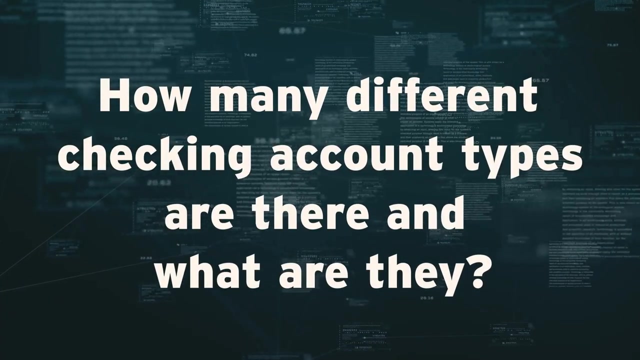 However, a closer look at the questions and options for overcoming the problems tells a much different story. Let's start with GPT-4.. It got only one question wrong. notice the air quotes on all three attempts. Here is the question: How many different checking account types are there? 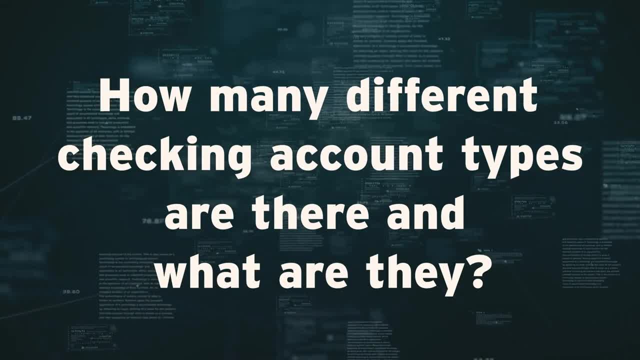 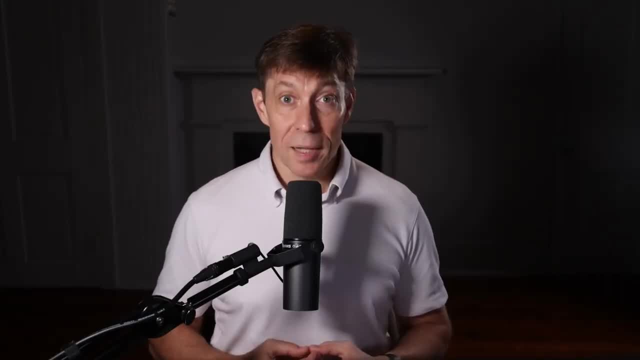 and what are they? A closer inspection of the response reveals ambiguity around the word type. When I slightly rewarded the question, which is what I would do as a user, it gave me the right answer. So in practice GPT-4 is closer to a hundred percent. Find also made errors that we 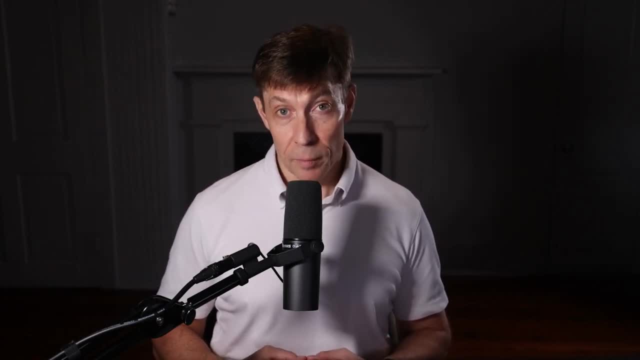 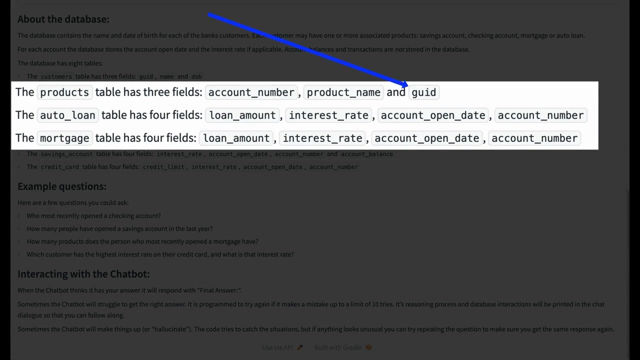 could correct with a few application tweaks or user behavior. It failed every time on the question: how many products does the person who most recently opened a mortgage have? for the same reason, The model fell into our messy data trap. It assumes the mortgage table has a user ID, when in reality 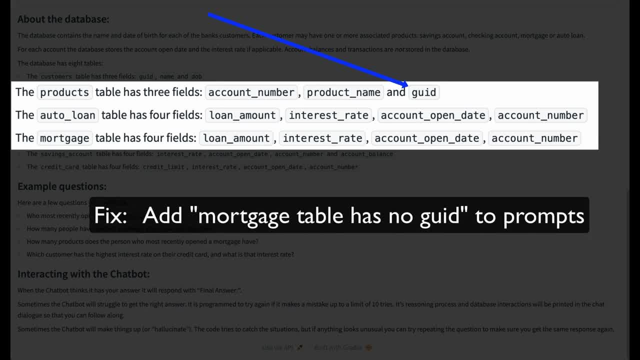 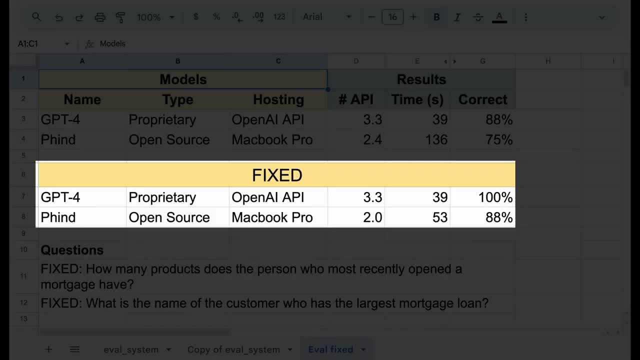 only available in the products table. Adding mortgage table has no GUID column to the prompt instructions solved the problem. So with these two quick fixes Find is looking much better. The speed is now comparable to GPT-4 and accuracy is up to 88 percent. I'm also confident I could. 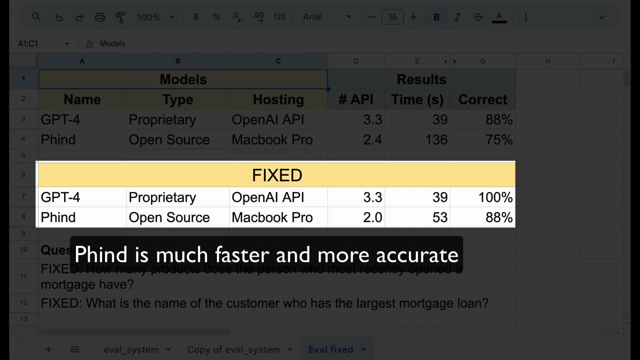 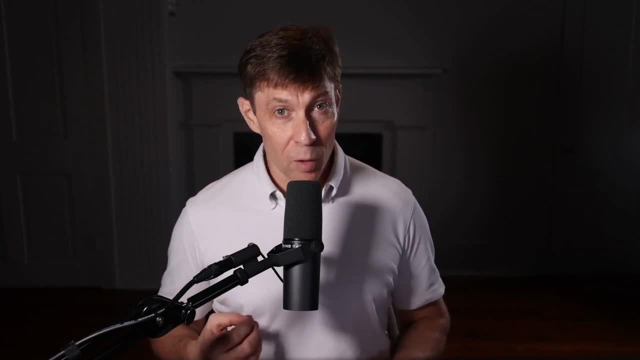 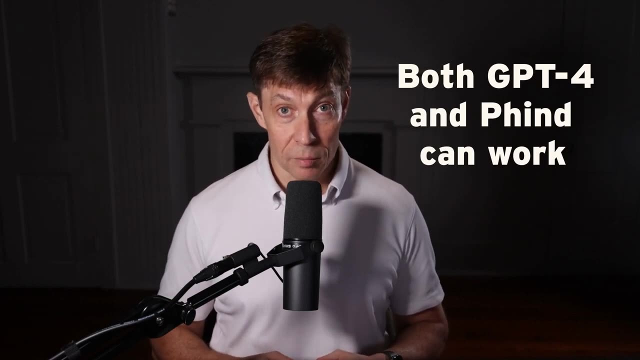 make a similar fix and get accuracy over 95 percent? These are just eight simple questions, so these metrics don't tell us a lot in isolation. The big takeaway is that both Find and GPT-4 can give good results when you customize them for your application. 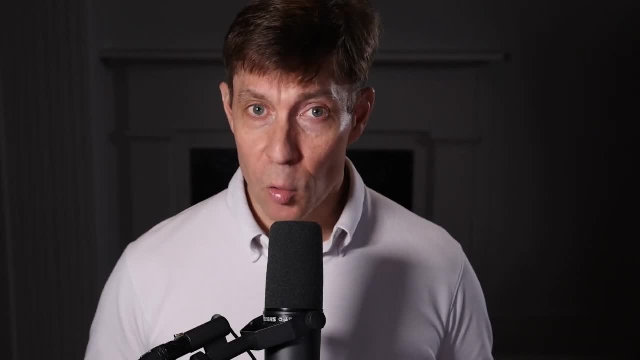 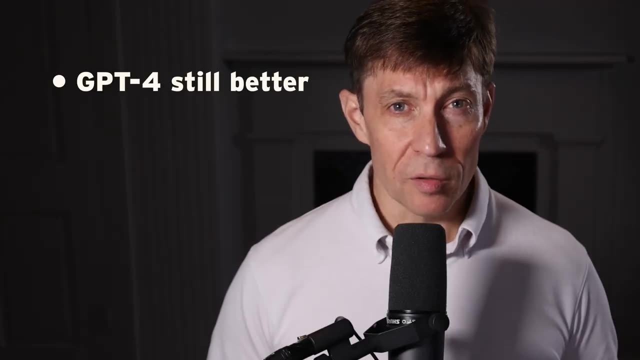 Let's now talk about what we've learned and what you should do. I'll start with your questions from earlier. Are open source LLMs as good as proprietary ones like GPT-4? GPT-4 is still better than open source models. It generalizes better across all tasks and still performs very 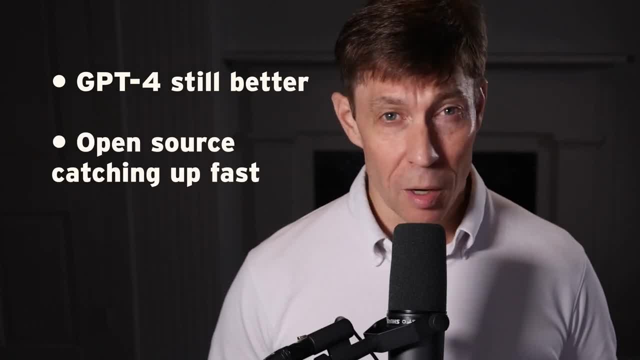 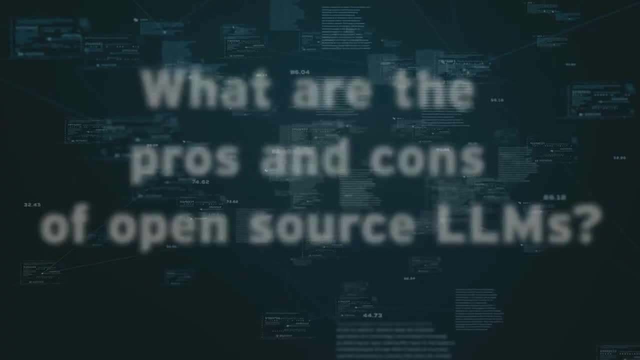 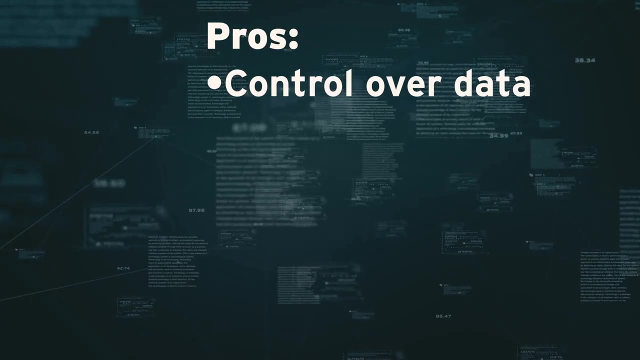 good at specialized ones. However, the open source models are catching up quickly and can be better and cheaper when customized for your task. What are the pros and cons of open source LLMs? For most companies, the biggest pro is that you retain full control over your data. Additionally,